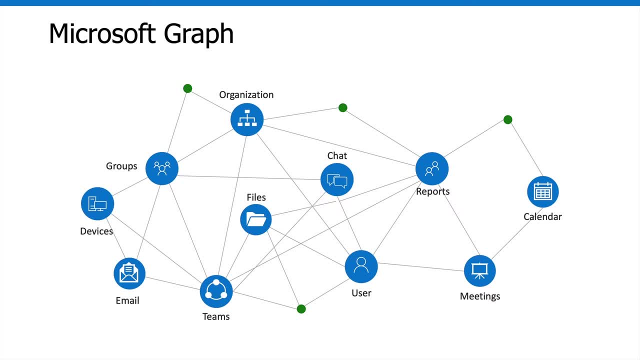 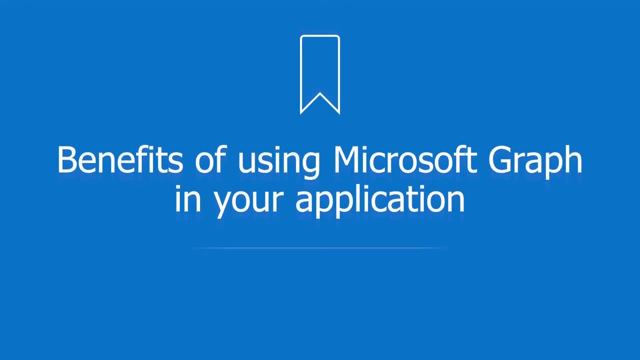 Well, Microsoft Graph provides an API to allow us to get to this type of data- and much more, in a very secure manner. To better understand the benefits of Microsoft Graph, let's revisit the customer application scenario mentioned earlier. The application needs the following functionality to enable: 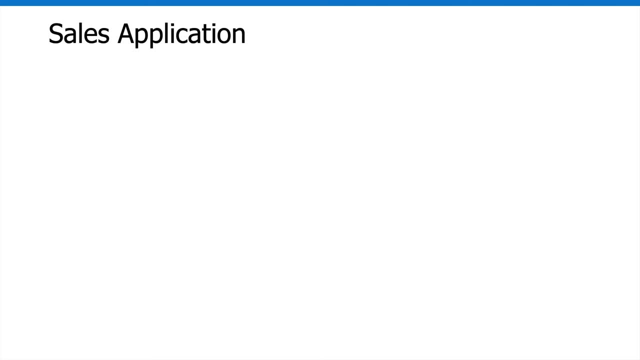 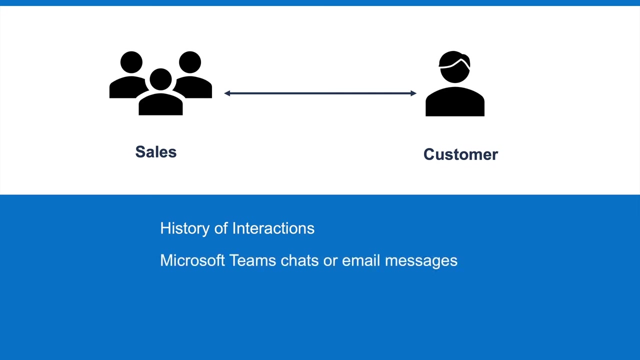 salespeople to work with customers more effectively. Namely, we might need email and chat meetings and notes, people and hierarchy within our organization, as well as files. Now, this could include getting a history of interactions between salespeople and customers through Microsoft Teams, chats or email. 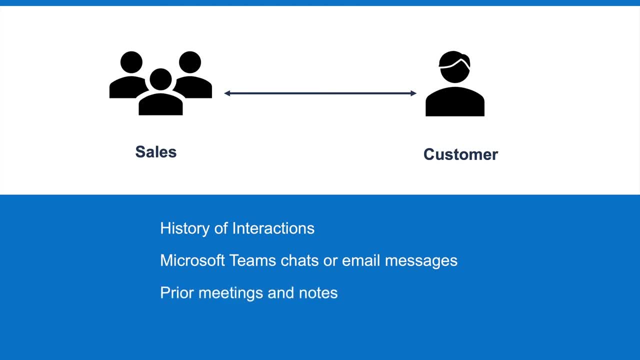 We might want to access information about prior meetings and notes, of course, and identify key people within the organization that can help out with customer questions. If we can access that type of data, we can pull it into our custom maps and get it where. 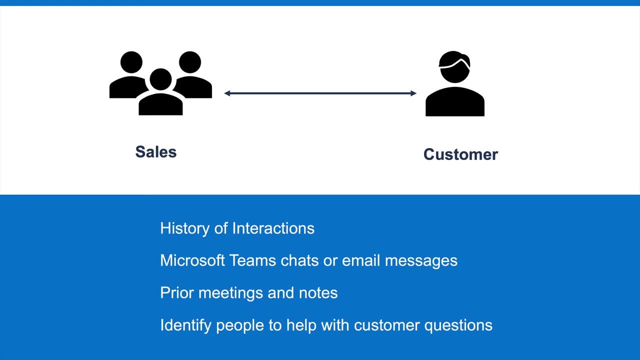 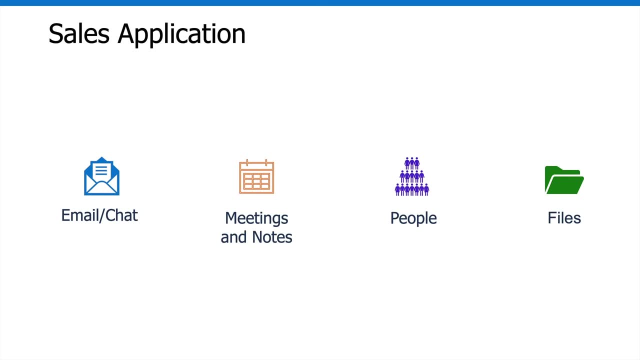 our users work every day, so they can make more informed decisions. Now you might think, well, couldn't I just do this on my own? Yeah, you could. in most cases, There's different APIs out there for Outlook Mail API. 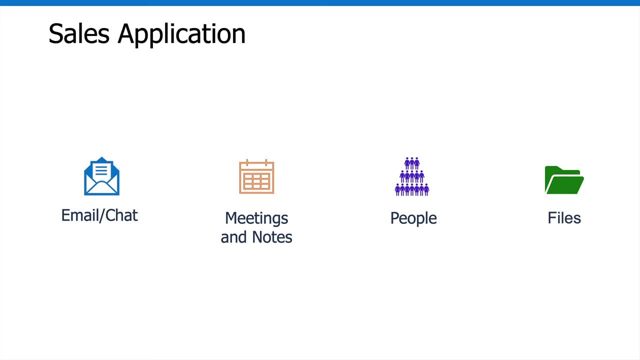 getting to calendars and meetings, or maybe the OneDrive or SharePoint APIs. but you'd need to learn all of that and as a developer, that means you'd have to have those individual skills and your team would have to have them, and that's a lot of APIs to learn. 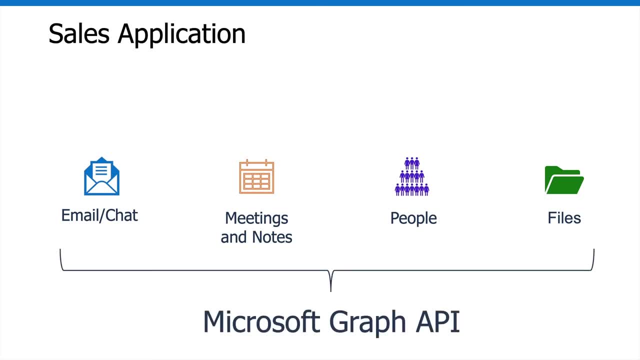 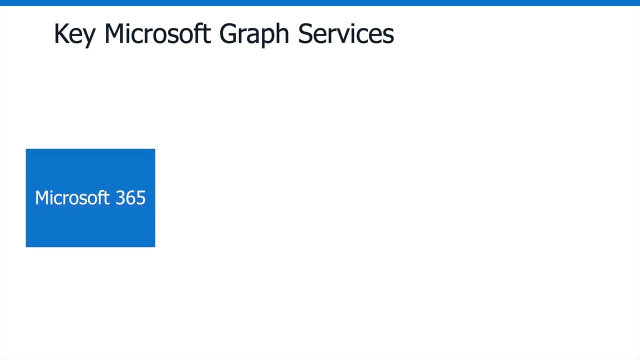 Microsoft Graph. pulls this all into a single, secured, unified API makes it much, much easier to work with. Now, as the sales application grows, it can include data from other services. We've talked about some of the Microsoft 365 data, but you can also get to Delve or Excel. 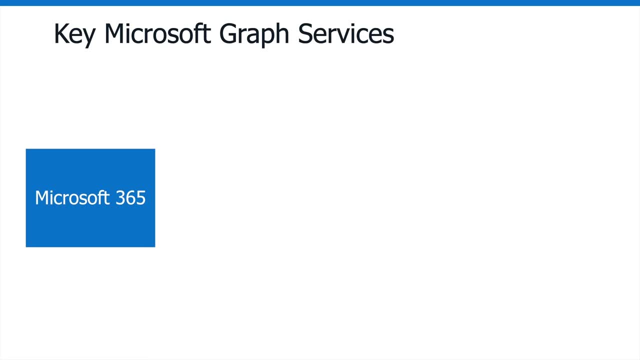 Microsoft Bookings, Microsoft Teams, OneNote, OneDrive, Outlook, Exchange- all of this and much, much more. You can even get to enterprise mobility and security services, such as advanced threat analytics data, advanced threat protection, Azure, Active Directory and more. 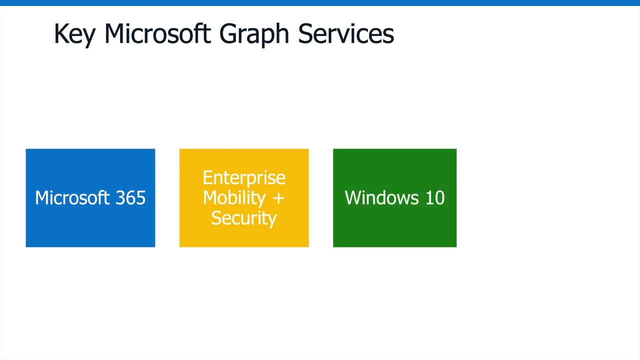 and even Windows 10 services. This can include information about activities, devices and different notifications, and then we can even tie in Dynamics 365 Business Central data as well. As mentioned earlier, security is a critical part of any organization, and Microsoft Graph provides built-in security to.